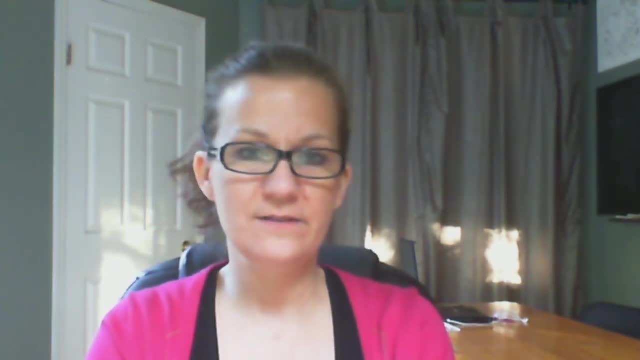 old enough You start understanding all this. You give them a weekly allowance of whatever $2. Doesn't matter what it is, And you start writing it in the journal. okay, And you only write in the journal when they're there with you And you're the only one that's allowed to write in the journal, because you're 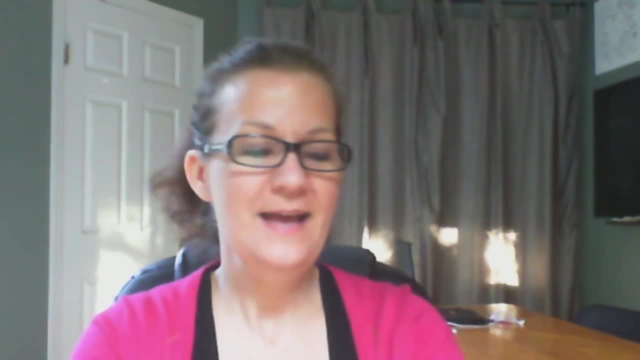 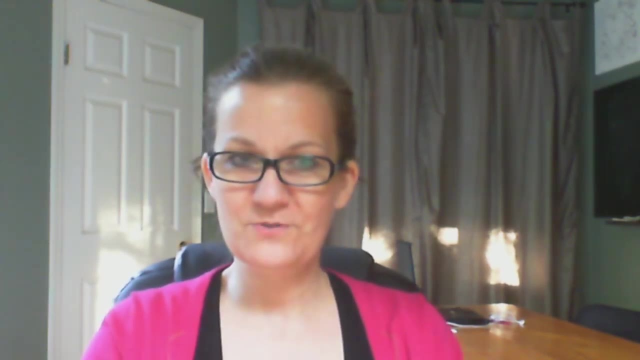 like the teller, right, But you're really. the gatekeeper is what you are, And all we're trying to do is to make them stop and think about every financial transaction, every deposit, every withdrawal, and watch their interest grow. You're providing them with interest. Figure it out as you like. I gave my kids 10% on every 100.. So if they reached 100, they got $10 interest. If they reached 200, they got $20 interest When they reached 1100,. 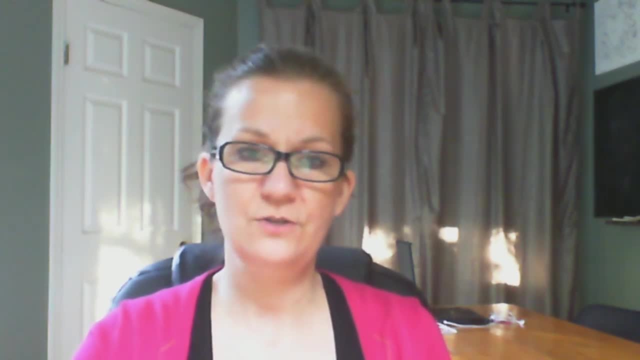 so when they got to 1,000, they got $100. But then I went back to 10% on every 100 after that. So then if they reached $1,200, they only got $20.. They didn't get 120.. They would have loved that. They only get interest on the same amount once. So if they spend money, they have to really work hard to save up and get rid of it. So that's what I suggest you do. So that's what I suggest you do. My kids became brilliant savers. Unfortunately, I didn't put this money aside. So when my son was 16,. 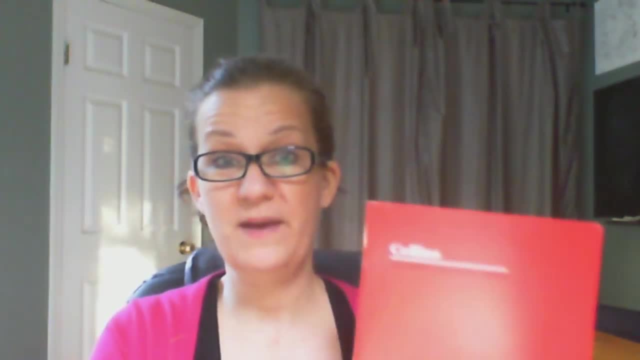 I had to write him out a check for what was in mom's bank, which was just paper and ink. I hadn't put it away, So I was up for thousands of dollars And I said to him: here's a check. You go to the. 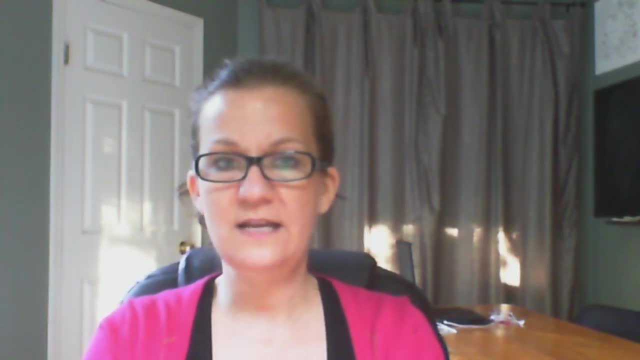 bank. You're on your own now- And both my kids- they're 20 and they're 15 now- They're both wonderful savers And they're also very thoughtful spenders. But the funny thing is they're also very 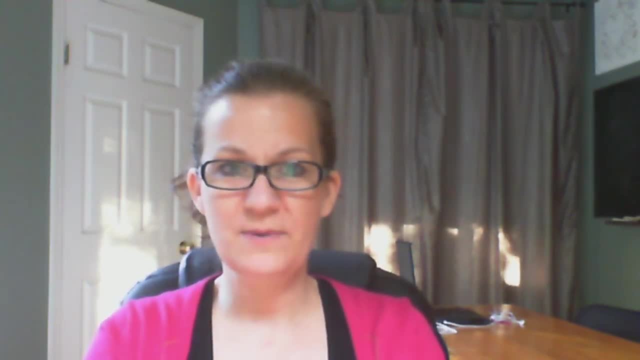 generous with their money. They're not just going to spend money, They're going to spend money on cheap, But they just consciously think about it. They spend their money where they want to And they always stop and think: And that's because of this mom's bank. Okay, it's a wonderful tool. 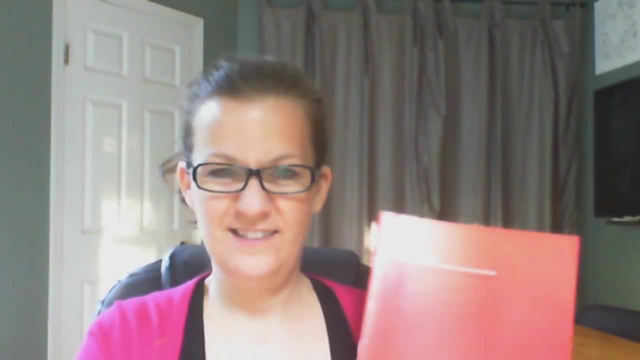 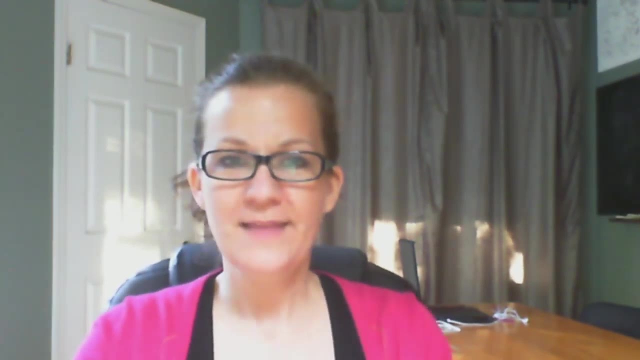 If you see me on TV with my little red journal and you see the anchor or the host laughing at me, just feel my pain with me. I love my journal. Anyway, good luck with that. Thanks very much for watching. Lisa Bunnage, Brat Busters. 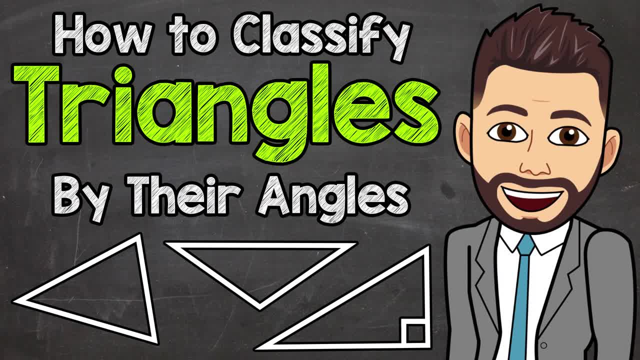 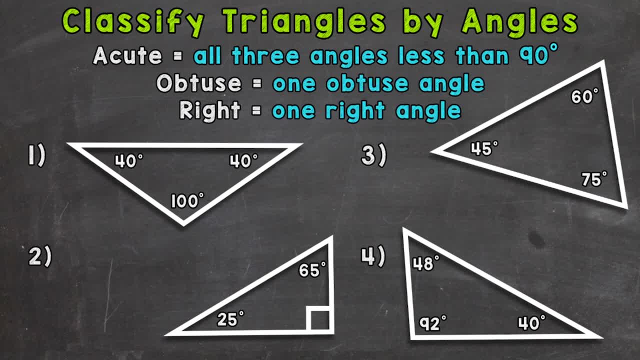 Welcome to Math with Mr J. In this video, I'm going to cover how to classify or name triangles based on their angles. Now we have three options as far as types of triangles based on angles, and we'll start with acute triangles. That means all three angles are less than 90 degrees. Then we